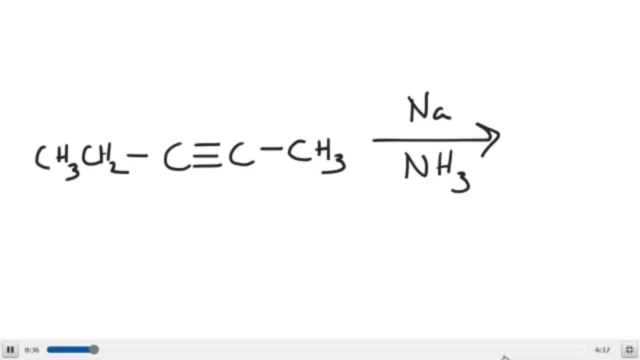 you don't seem to think that it's NaNH2.. We do not want NaPy, NaPy plus, That is a different version of sodium That's got its electron removed. We want the sodium that has the electron And that's absolutely critical that the sodium 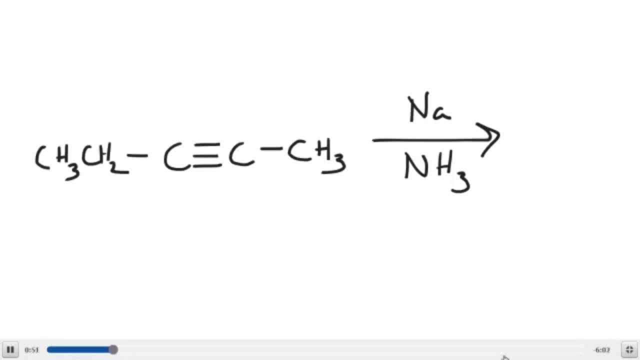 has its electron. Now I'm going to, on the next slide, draw this triple bond in a different way, so that we can see the orbitals and where the electrons are in those orbitals. It's very critical because you need to remember that orbitals can have none, one or two electrons. 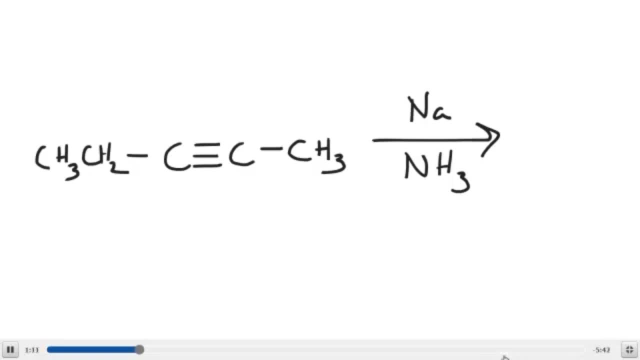 So I'm going to try to show things with orbitals on top and on the bottom to show the electron pushing mechanism. So if I want to see this with orbitals, I'm going to draw out the p orbitals on this carbon system. One of them I'm going to draw in blue, The other one I'm 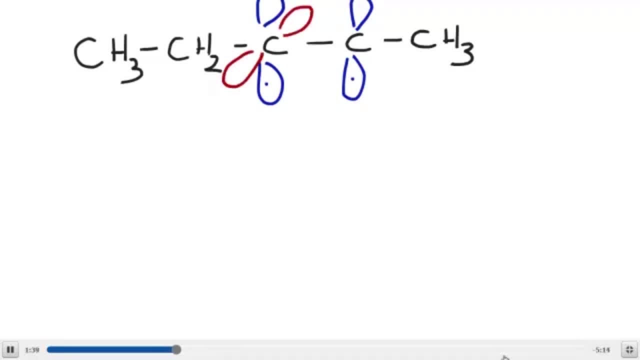 going to draw in red. The other one should be coming in and out of the page at you. I just can't quite draw it that way. Okay, But that would be the triple bond that we're talking about Again, the same way of looking at that in our normal convention for mechanisms, which is to be: 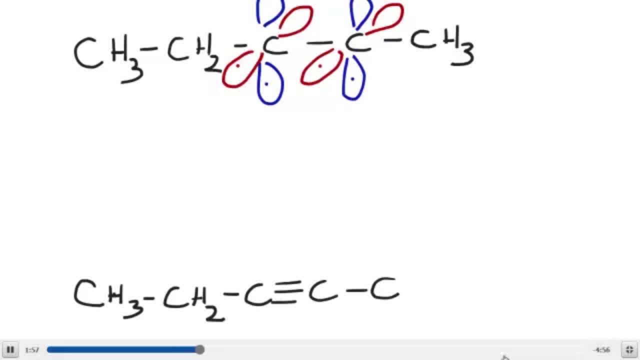 showing that triple bond here like this. So I want you to be aware these mean the same thing. Now sodium- I'm going to draw it up here on the top- has one electron. So it's one electron in its valence shell. If you're just using Na, it's very important, you realize. 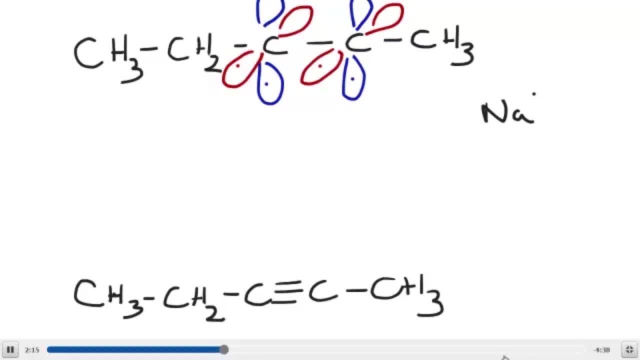 that it has an electron. The whole reason you normally see sodium as Na plus is because it likes to get rid of its electron, And that's what it wants to do in this case. It wants to dump off its electron somewhere. I call it the dump off my baby electron syndrome. 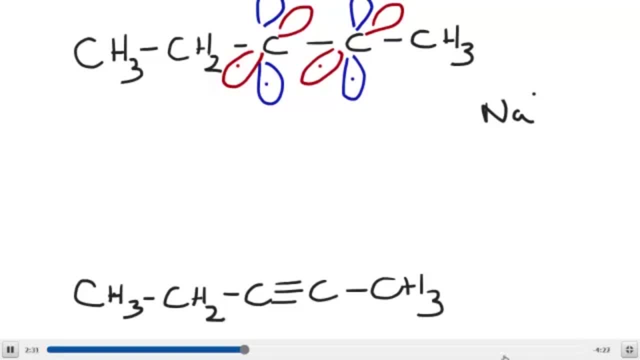 We don't want our baby electron. Somebody else is going to have to deal with it And it doesn't matter which of these four p orbitals gets it. but somebody's going to take baby electron And it's one electron, so you use a single-headed arrow to show its movement. So if I'm doing 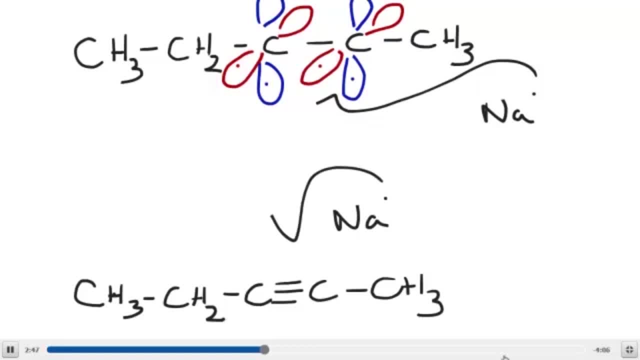 it down here. okay, I'm going to show somebody taking it. As a result of that, a pi bond is going to break. So one of these electrons pairs up with it, the other one hangs out by itself. So you're breaking a pi bond. So I would show that here, with one electron going. 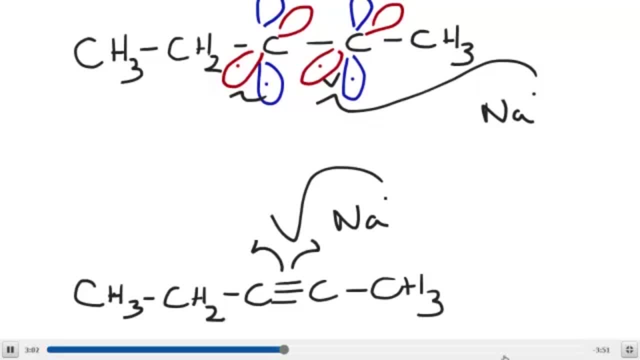 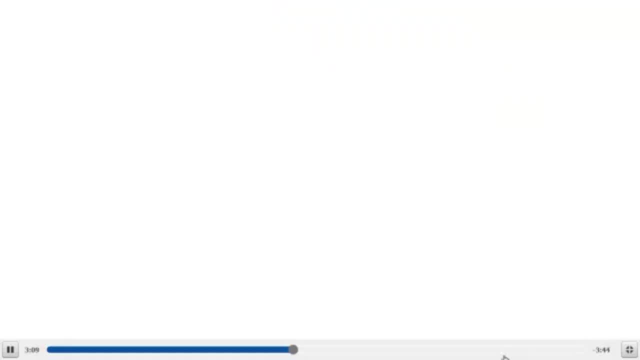 one way and one electron going the other way, because you're breaking the pi bond. So if it's going to change the hybridization of these carbons, okay, I am going to draw in the double bond at this point in time. But these have now become sp2 hybridized And 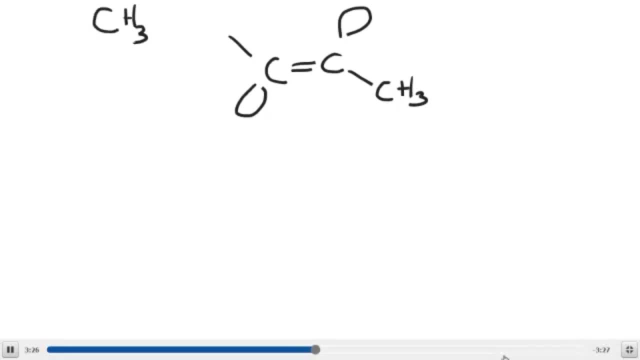 they want to get as far away from each other as they possibly can due to electron repulsions. Now we have an Na plus over here. okay, Subtitles by the Amaraorg community. If you want to draw it this other way, it's just fine. I'm just drawing the same thing. 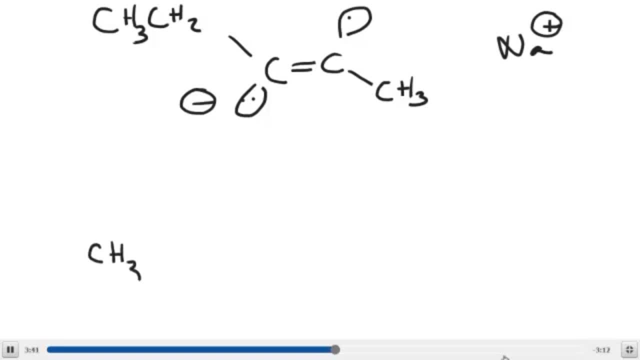 above and below. Take one right there and two there. This is called the radical anion, But these carbons, literally, are now sp2 hybridized. due to the fact that we dumped an electron into one of those p-orbitals, It changed its hybridization from a p-orbital to an sp-2. 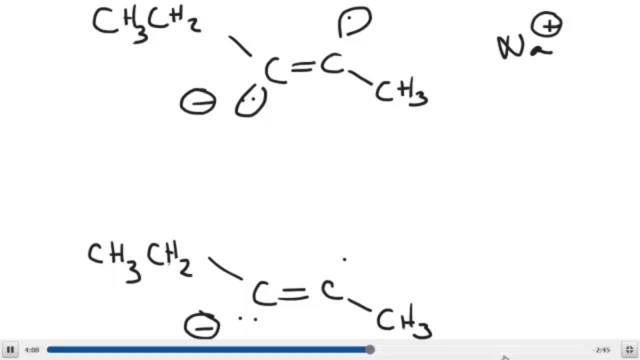 hybrid orbital Subtitles by the Amaraorg community. http//wwwu. e-mailtestwith- Fallon號wishesblogspotcom. 2017 got a negative charge Now if you look at your pKa table and look at the bases, because 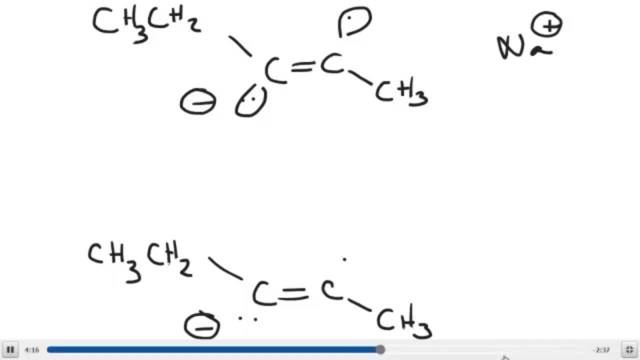 this is a base. now it's got a negative charge. This would be the corresponding conjugate base of an alkene. If you look at the pKa of an alkene, it's around 45.. They're terrible acids, So this is a fantastic base. I mean it is awesome. There's only one base stronger. 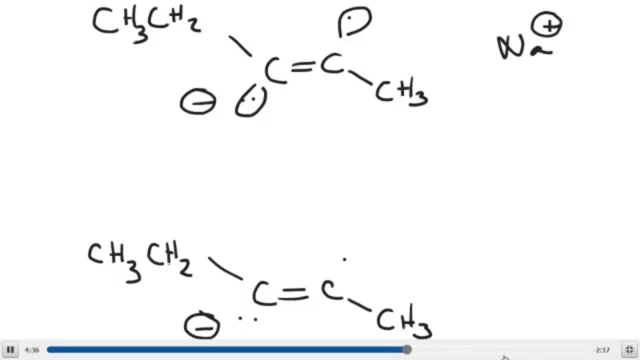 than this, and that would be a deprotonated alkene. So this is an awesome, awesome base, And our solvent here is ammonia. Normally, ammonia is never an acid, But in this case its pKa is such that it's going to be a proton donor. Ammonia has a pKa of 36.. So this is 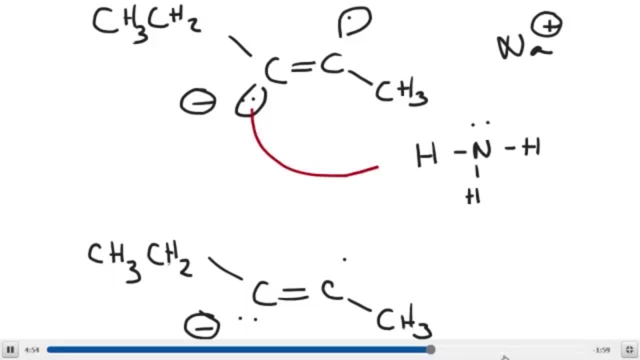 favorable acid-base chemistry, This pair of electrons will come in here and take the hydrogen and as that happens, the hydrogen-nitrogen bond will break and nitrogen will take those electrons with it. And I am using double-headed arrows here because this is two electrons that are moving And 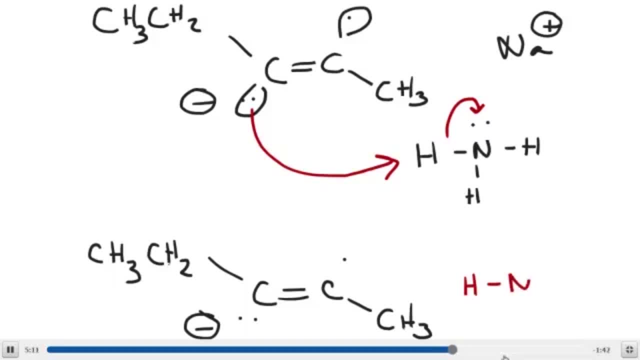 you can again do this from the bottom as well. It's just as good. So if I want to do it here, just take the hydrogen, give the electrons back, All right. so what do you get as a result of that? Well, you're going to make a radical. Okay, we still haven't taken care of that. 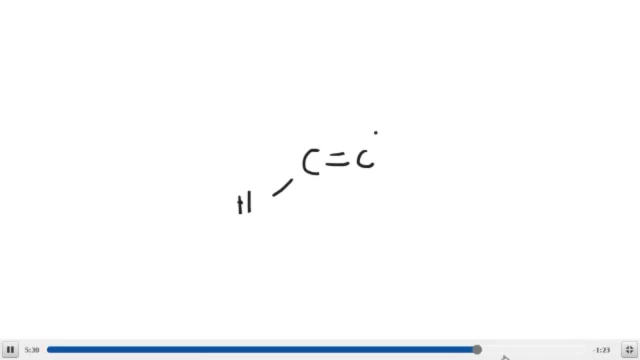 radical. but we've now given ourselves a hydrogen in one of these locations, And the reason this doesn't ever do anything is that it's going to make a radical. It's going to make a radical, but it's not going to do anything. but what I am showing you is because you still 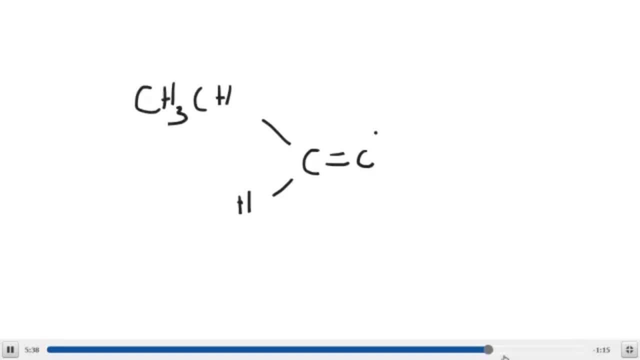 have a pi bond. You cannot rotate pi bonds, So they're stuck in place. once this has occurred, It doesn't have anywhere else to go. But it's still a radical. It needs other electrons And there are more sodiums in there, So another sodium comes in and says: hey, you can have. 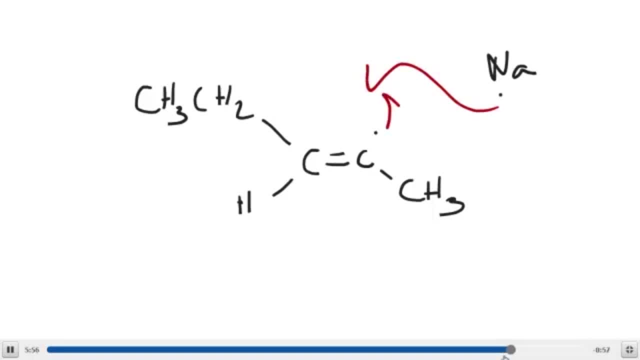 my electron and we can be buddies. So we're going to be buddies. As a result of that, we make another anion And it is again the corresponding conjugate base of an alkene. so it's a really really. 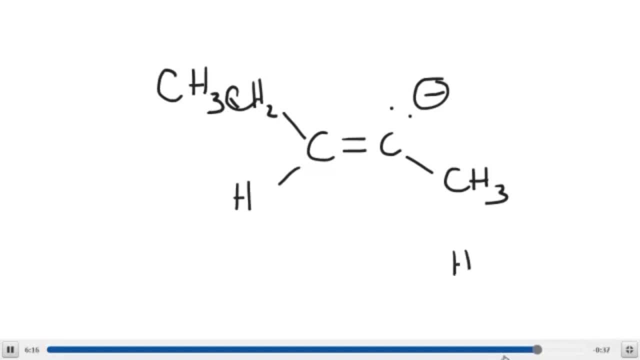 strong base And our solvent in this case is still ammonia. Okay, there's the sodium hanging out there to balance charge, But this guy is a strong enough base that he can remove the hydrogen off of another ammonia solvent molecule. And at the very end you have made a trans-alkene, because you can't rotate that pi bond. 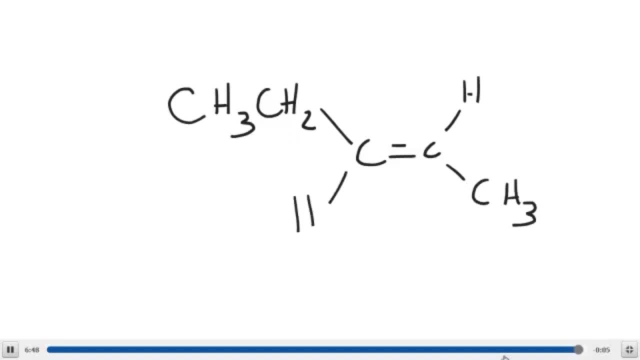 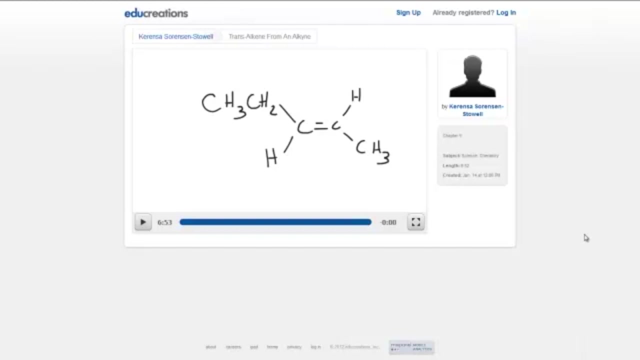